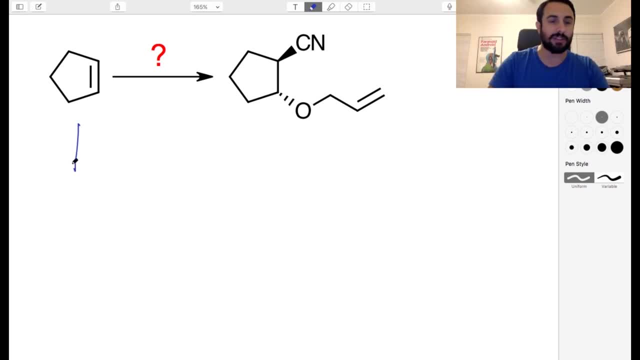 that oxygen functionality that we want. So why don't we do this? Let's do MCPBA. That's just the classic. the metachloroperoxybenzoic acid is the classic reagent for epoxidation, So let's go. 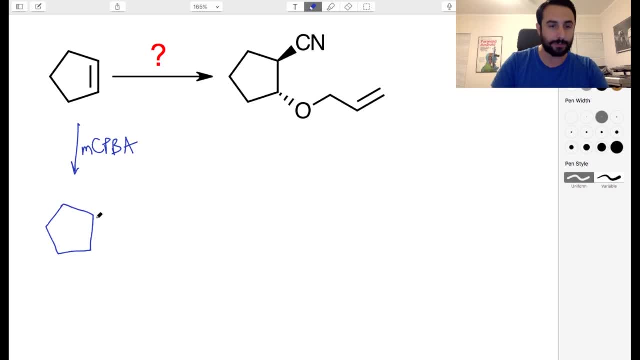 ahead and do that And we'll say that we'll put that on the dash. And so now this would be a great opportunity to go ahead and introduce the nitrile, because we know that we've got a great SN2 nucleophile right. 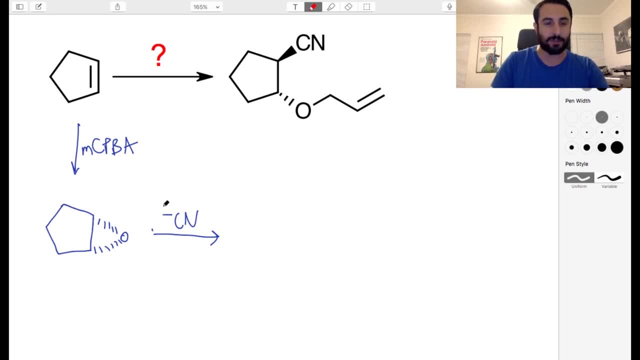 And so this is where a lot of the important chemistry can occur. If we have this attack here, right, we're going to do that, And let's just say it picks up a proton from solvents, So we're going to get our hydroxyl, So let's put the CN there, And then 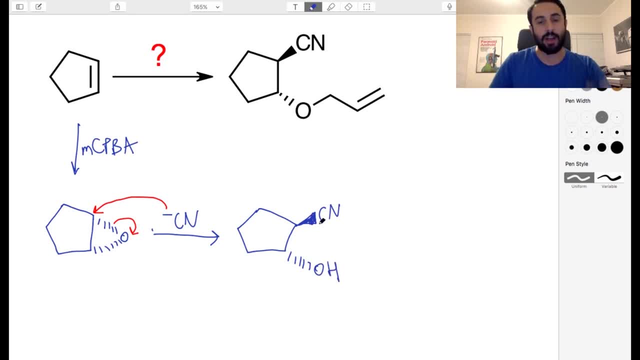 we've got OH right Now. so a couple of things here. We know that SN2 proceeds via a backside attack, So we know that this has to approach from the top and then kick this over here. So that is where the trans-stereochemistry comes into play here. So now we're pretty close. We just have to. figure out how to get this alkyl from here. So we're going to do that, And then we're going to do that. So we're going to do that, And then we're going to do that, And then we're going to. 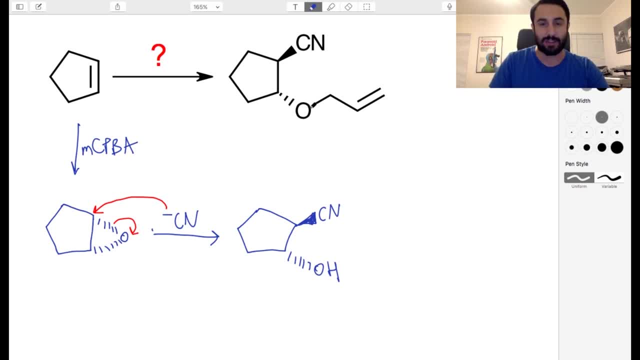 So we want to go from a hydroxyl to an ether. We can see that this oxygen here is already present on the molecule, So we're going to want this oxygen to attack something. So to me, Williamson, ether synthesis is the very obvious choice here, because we know that we can just deprotonate a 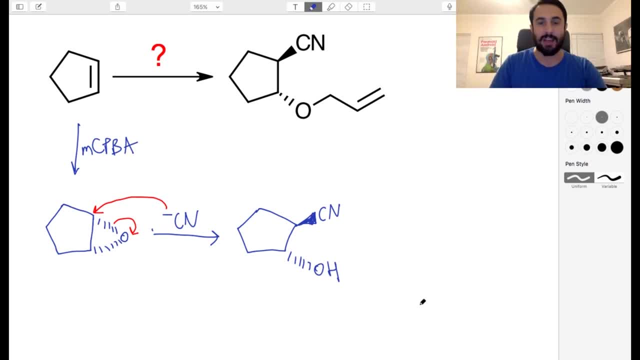 hydroxyl, and then have that do SN2 on some alkyl halide and we're going to be good to go, And this alkyl fragment certainly can have come from an alkyl halide. So let's just deprotonate. So 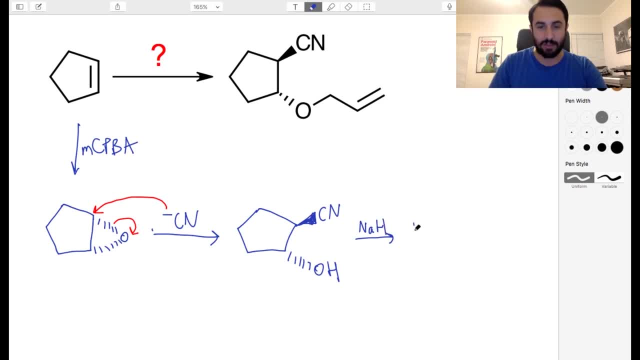 let's do. usually, sodium hydride is probably going to be the classic reagent used to prepare the reagent, And now we have the alkoxide. So with the alkoxide, now we just need for this to attack this vinylic bromide, right? Because if this attacks here,